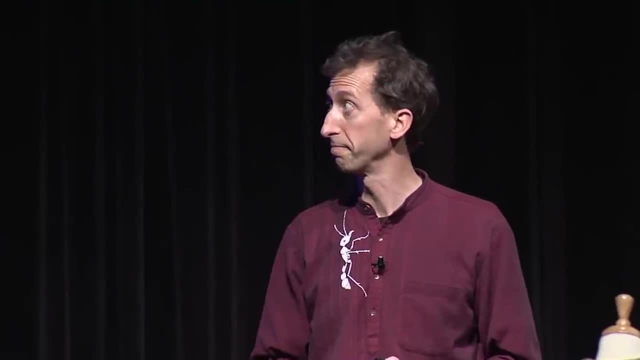 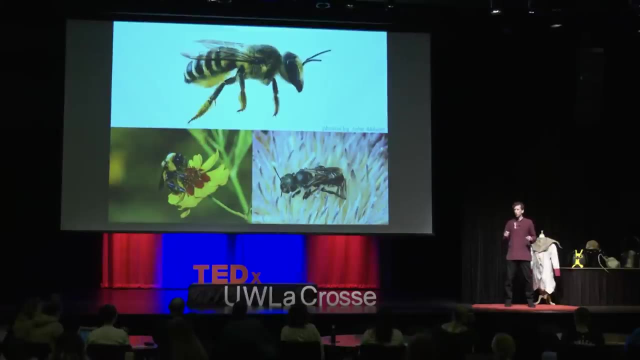 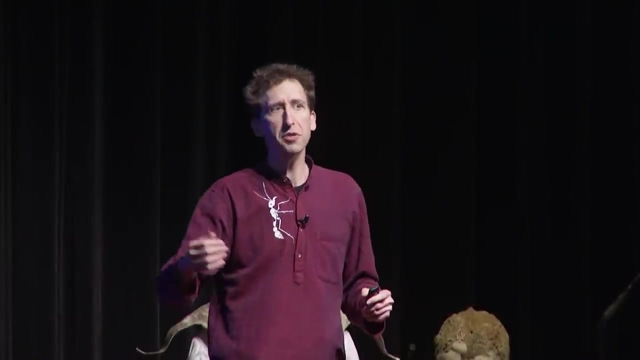 On which we depend, Like pollination. Every third bite of food you consume you can thank an insect pollinator, for They transport pollen from a male anther to the female stigma of flowers, facilitating reproduction in flowering plants. Insects also disperse seeds and nutrients. They aerate the soil, They'll decompose carcasses and dung. Insects also serve as food for well, think of your furry and feathered friends, which largely depend on insects and their diet, As have we. our ancestral hominids most certainly incorporated insects in their diets. 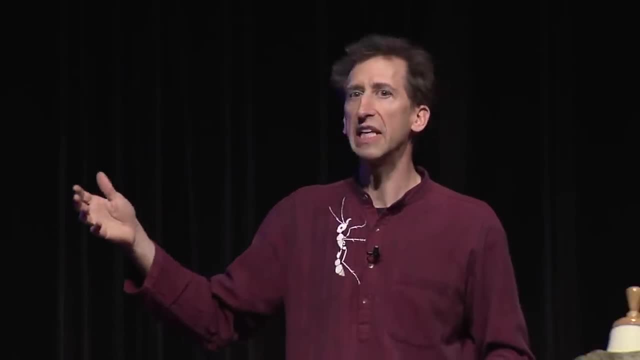 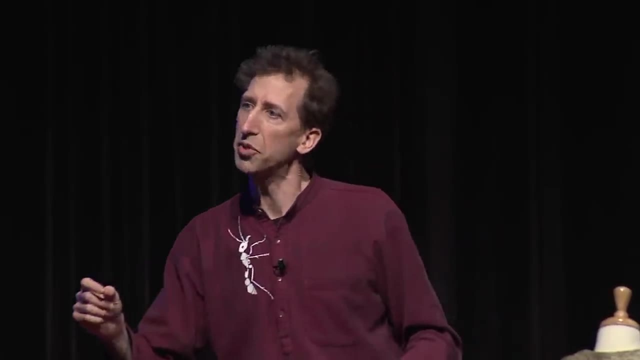 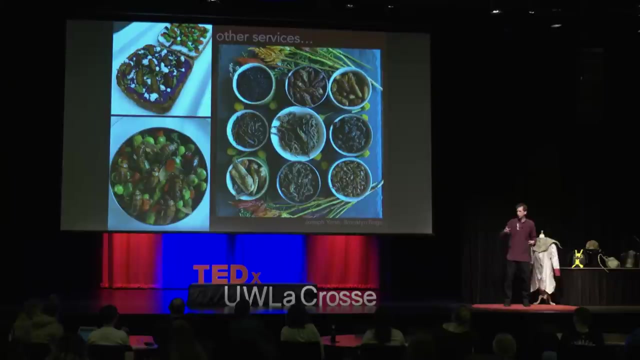 And today, entomophagy: the practice of eating insects is growing and growing, In no small part Because insects represent a far more sustainable source of protein than a cow or a pig. So, along with ecological services, we can think about cultural services. 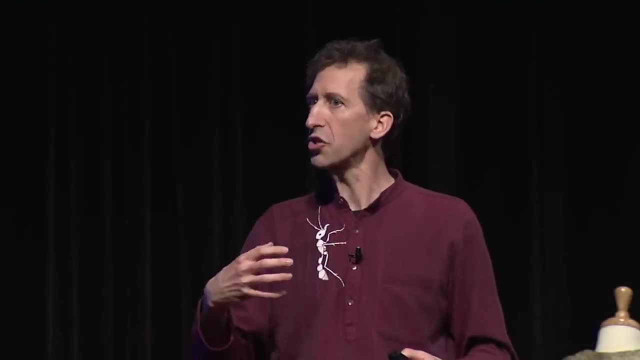 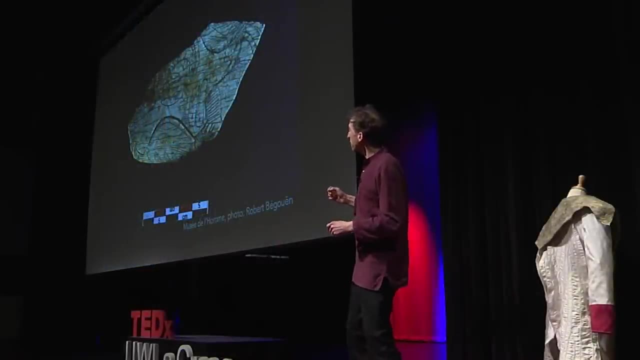 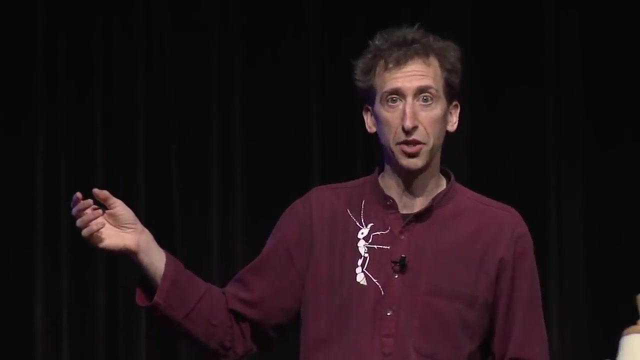 And I believe that insects have largely made us who we are by shaping our cultures. Fifteen thousand years ago, an artist in a French cave inscribed this image of a cricket on a scrap of a bison bone, Possibly the oldest depiction of an insect by a human. 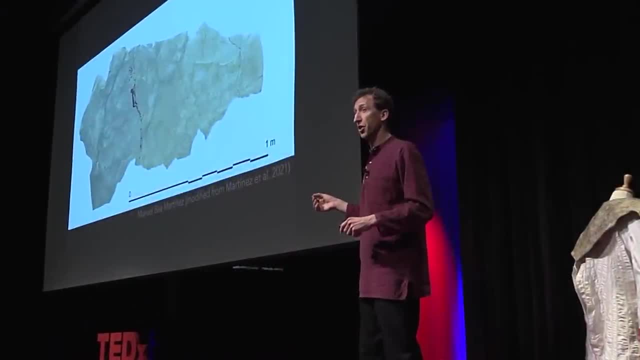 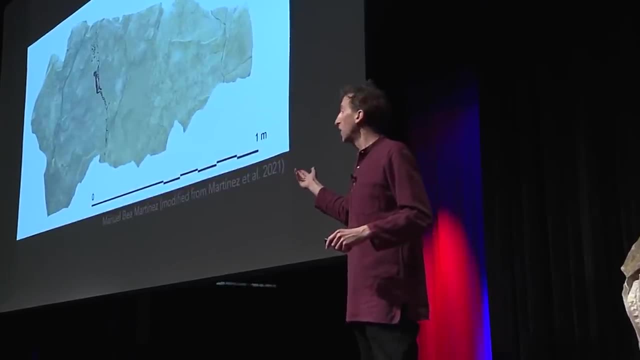 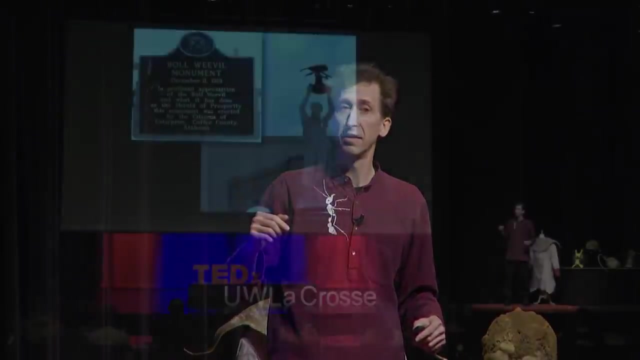 Also thousands of years ago, in caves in Africa, in India. at this newly discovered cave site in Spain, you find paintings of humans robbing honeybee nests. Insects serve as food for well. insects serve as symbols and have throughout history and across cultures. 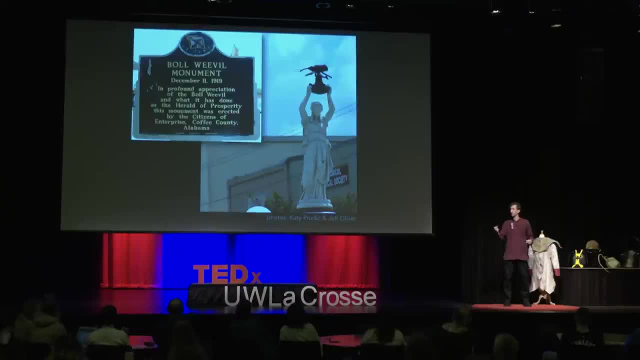 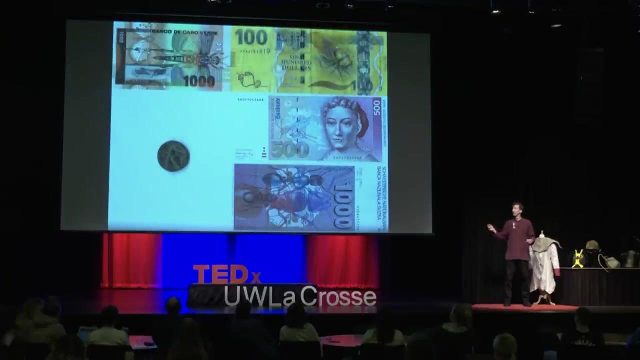 Think of ancient Egyptians worshipping the sacred scarab beetle, And today, in Alabama, denizens of enterprise hold aloft as the herald of prosperity a boll. weevil Insects are found on our currency alongside the face of Maria Sibylla Marion. 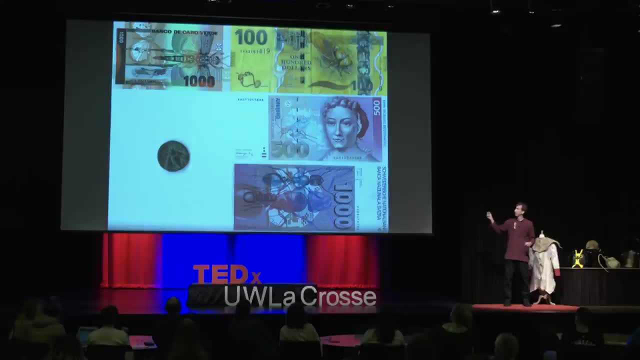 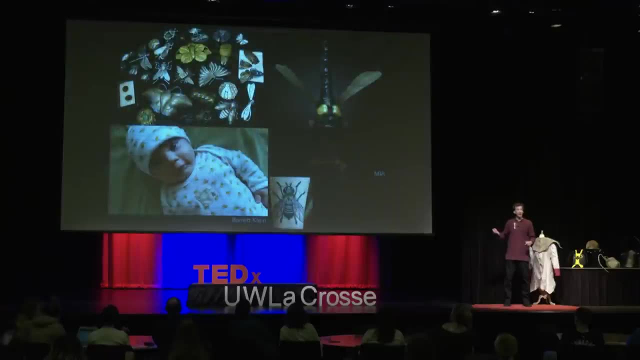 a pioneer of entomology, And on our planet and on our postal stamps, And on our bodies, whether it be a tattoo, samurai helmet, jewelry or bees on Riven's body. My son And I'll take this opportunity. 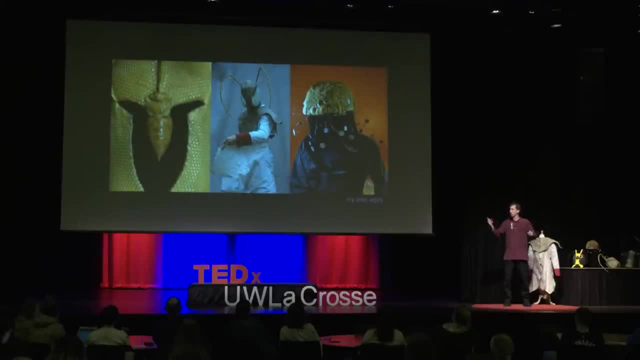 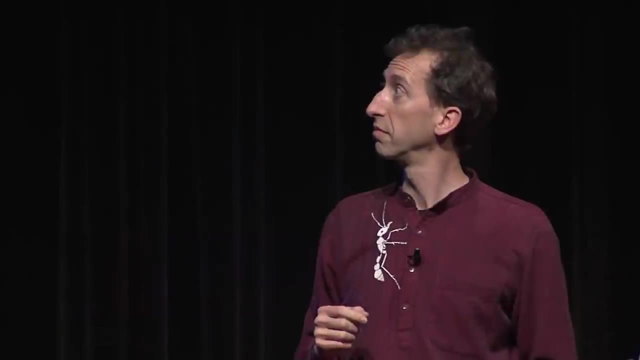 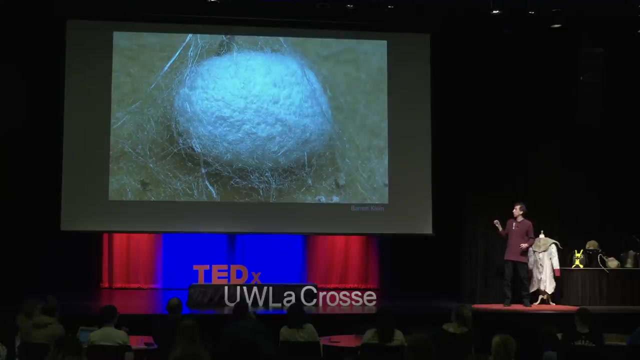 this platform to reveal to the world some of my secret identities. in the garb produced from insect products Like silk, This cocoon was spun by a single caterpillar, a bombix mori, silkworm moth. This was a prized commodity. 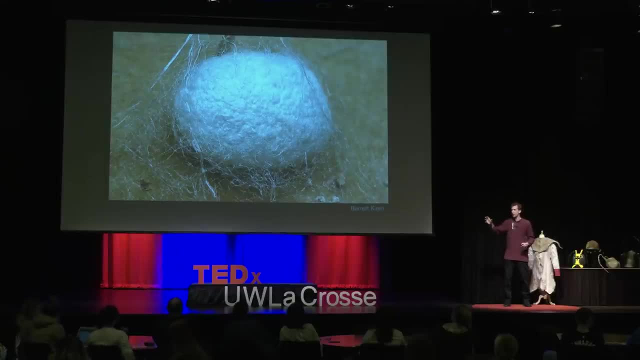 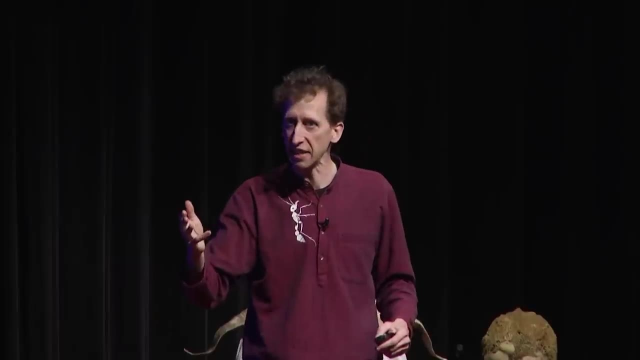 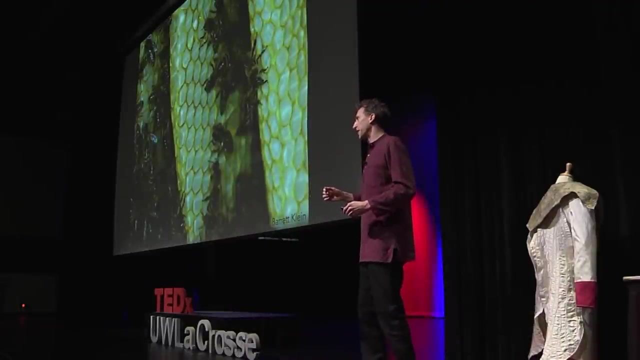 that brought swaths of the world together with a silk road. But not only commodities were exchanged: language, culture, religion, ideas transformed the world. Beeswax- Think encaustic. paintings, Candles, Adhesive. All thanks to honeybees, Which also provide honey, of course, and propolis collected from tree resin, Cochineal extract. Pulverize these scale bugs and you'll find a scarlet dye that the Aztecs used and the Spanish conquistadors monopolized. 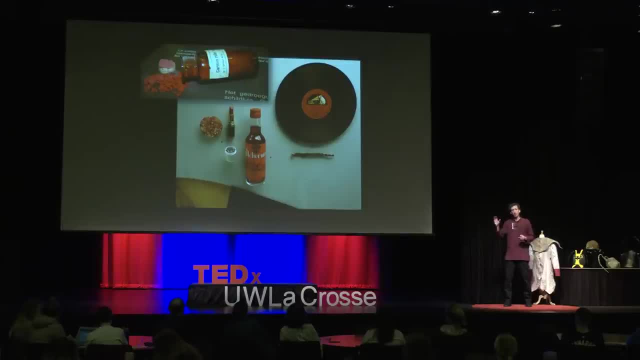 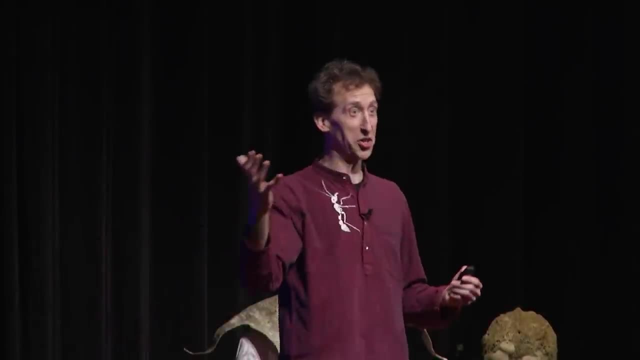 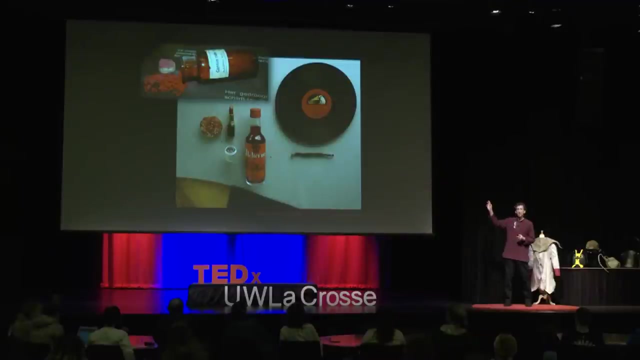 that changed the world in terms of a rare organic form of bright red, And maybe some of you are wearing cosmetics or consuming food or drinks dyed with the bodies, the pulverized bodies, of cochineal bugs On the right shellac from lac bugs. 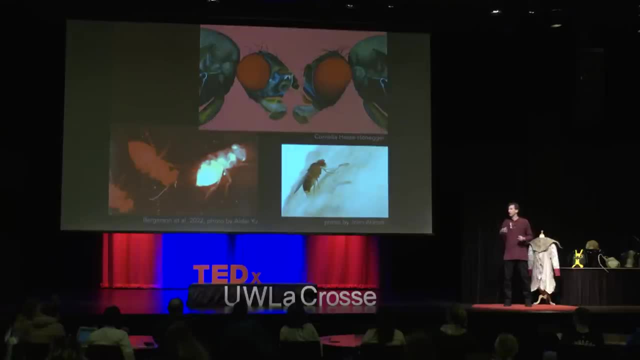 Insects inform us. We can learn from insects. For example, this species, Drosophila melanogaster, fruit flies, are a model system. Why? Because we share many of our genes with them, So we can understand better how we operate. 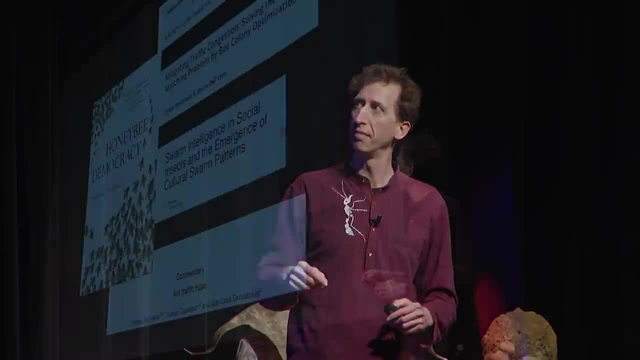 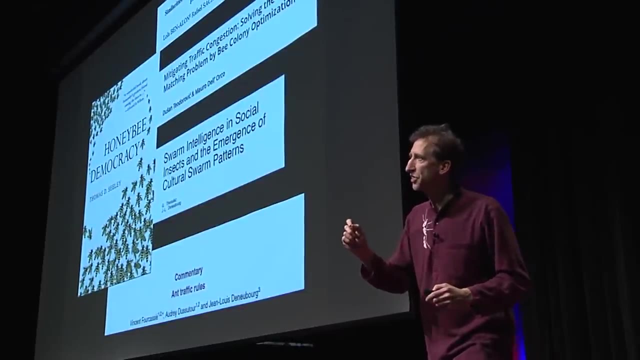 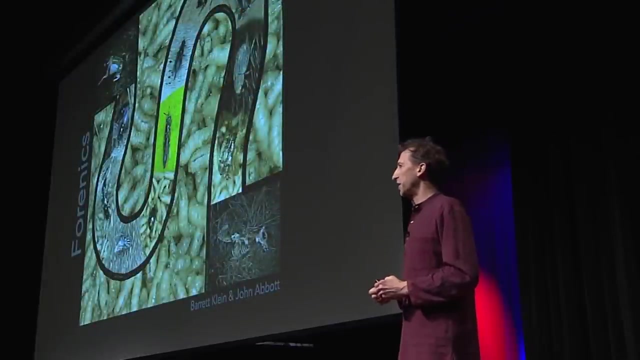 by looking at how they operate. We can also look to insect societies. How do they regulate traffic? How do they make decisions? Can we learn from those decision-making properties or processes? We can solve crimes through forensic entomology. So look at the species of insect. 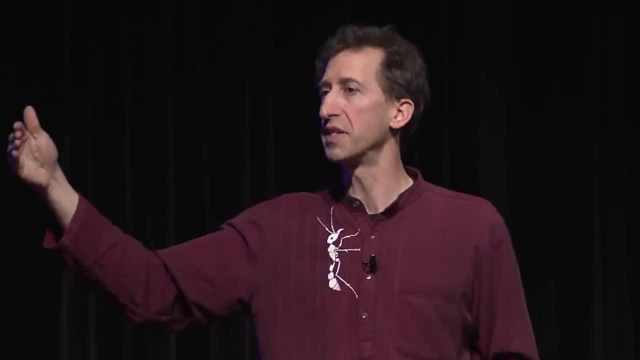 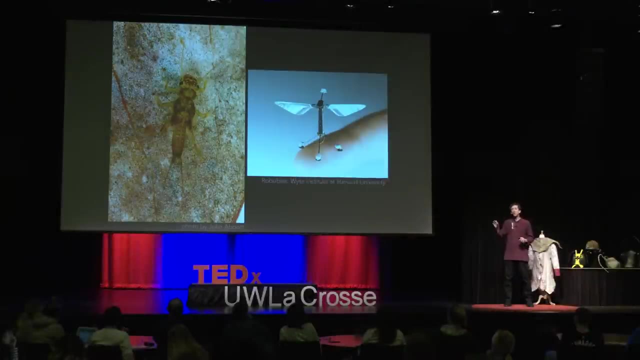 on a corpse and the stage of development of that insect, and you can date back time of death. We can use insects as indicators, bio-indicators, say the health of streams with that insect on the left, Or we can mimic insects. 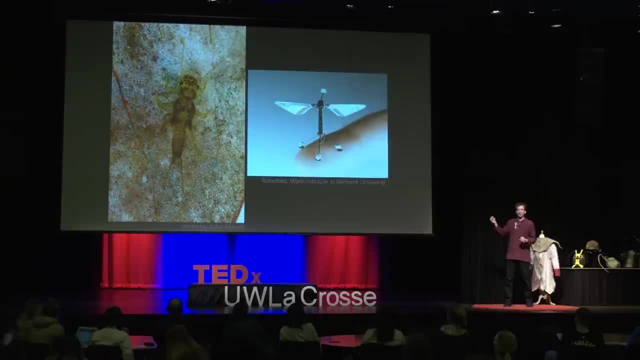 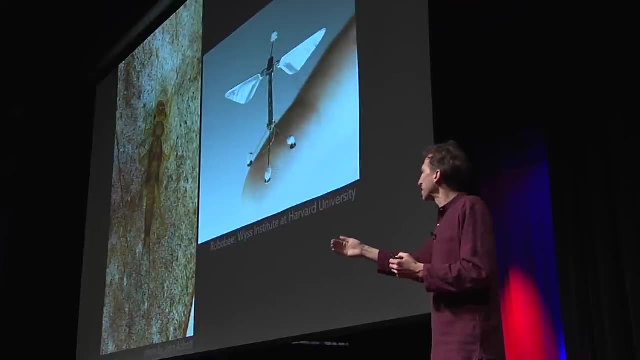 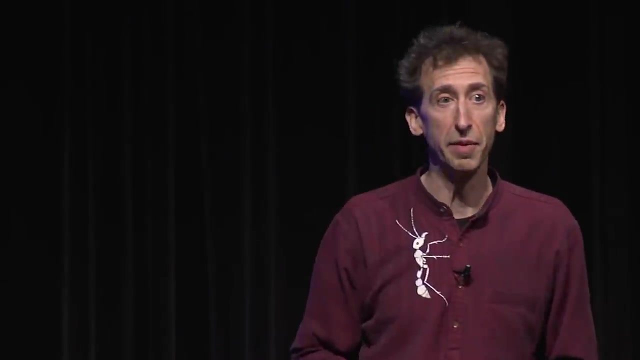 in terms of their amazing flight capacity. This Robobee, built at Harvard, is what might come to pass as a means of investigating danger zones. There are other ways to mimic insects, say through dance. Louis Fuller in the late 1800s. 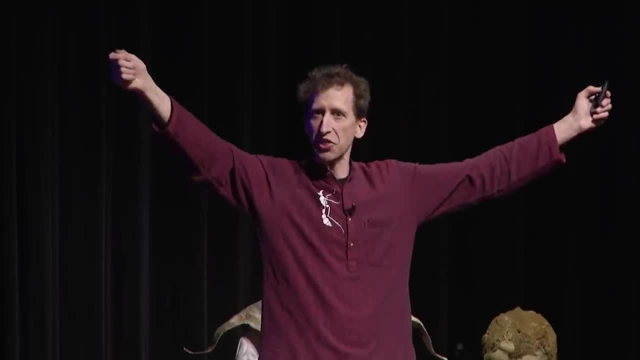 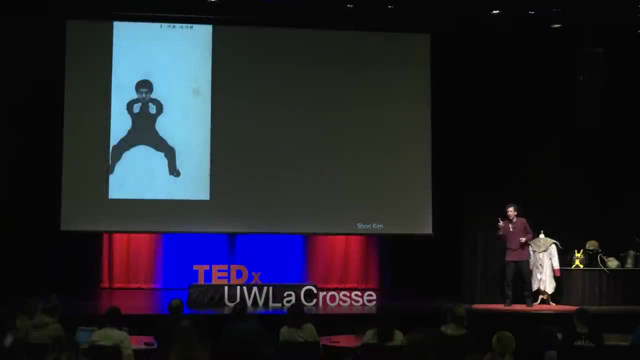 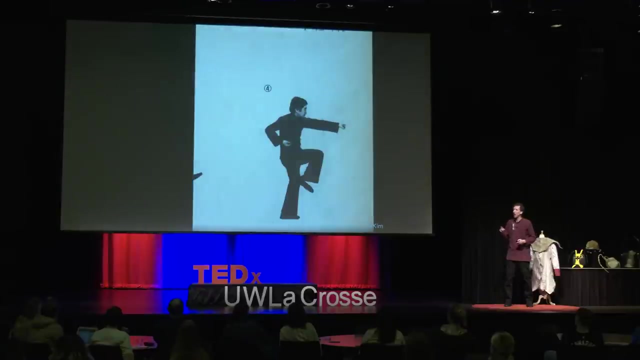 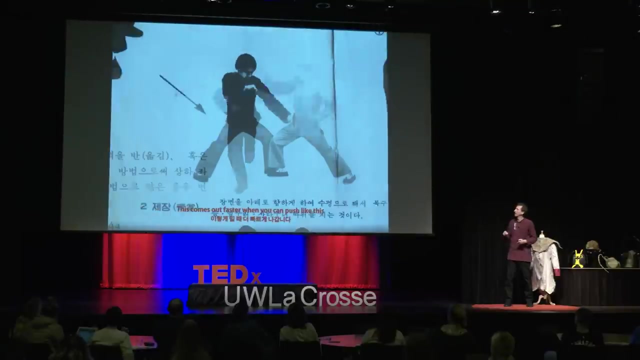 produced the butterfly dance by extending her silk dress with bamboo rods. Here I challenge you to identify the insect that this martial artist in an animation by Shown Kim is mimicking: Hint. look very carefully at his arms. Mantis-style kung fu. 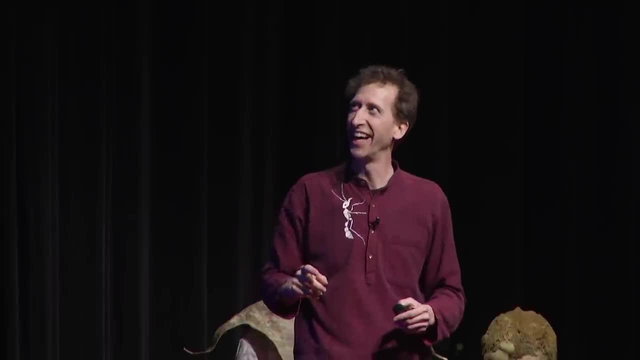 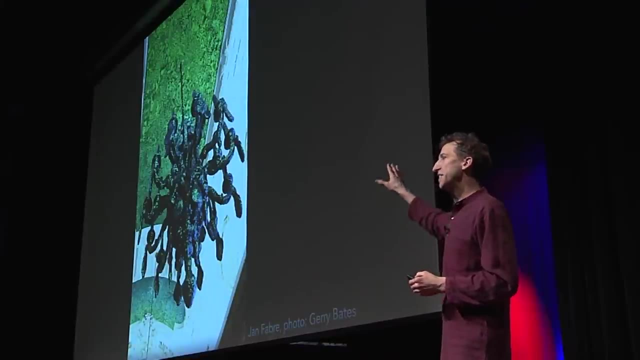 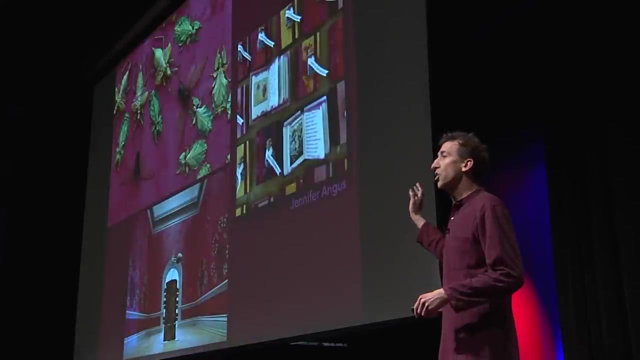 Anybody get it. Visual arts: A wealth of insects incorporated On this ceiling and chandelier in the Royal Palace in Brussels, Belgium. a million elytra and the front wings of metallic boring beetles shimmer The walls of this hall. 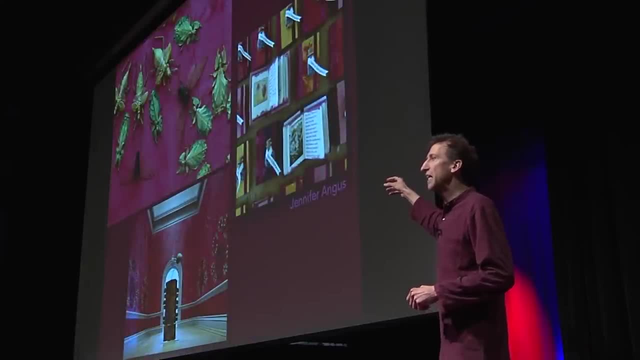 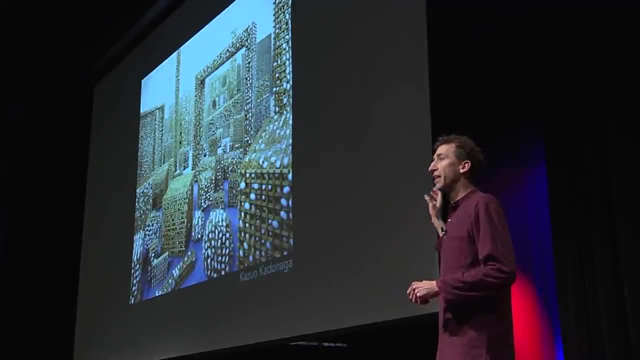 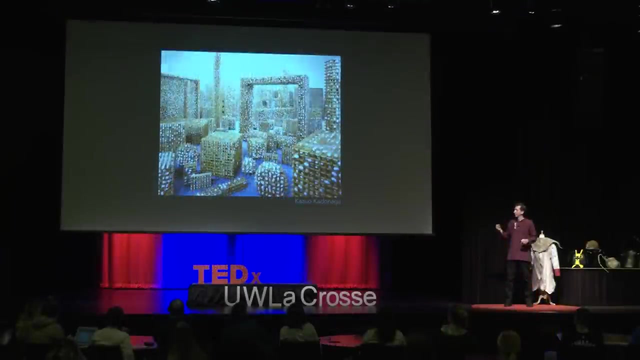 and those Insect Dreams. books laden with cochineal extract. thanks to Jennifer Angus, Kazuo Kadanaga produced this cityscape of 110,000 silkworm cocoons. Artists will sometimes collaborate with insects. Hubert Duprat takes caddisflies. 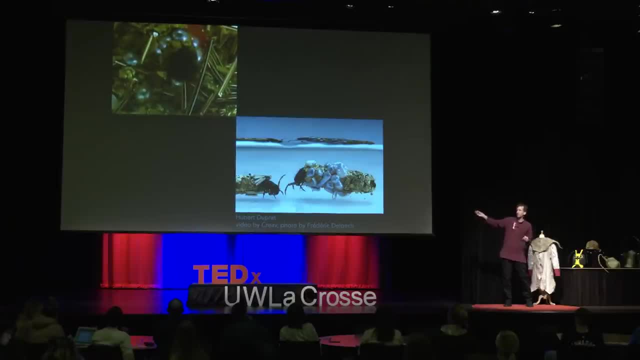 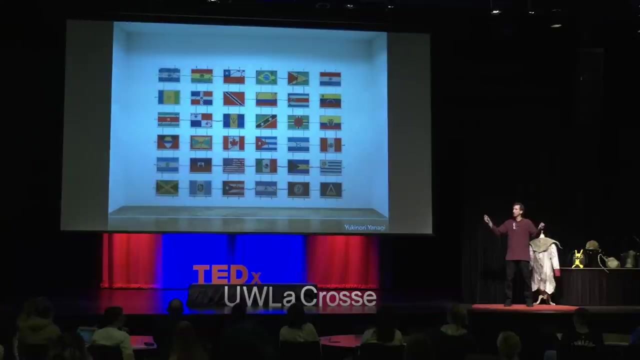 who would normally build their protective cases out of sticks and stones, and offers them gold spangles and pearls. Yukinori Inagi invites ants to disperse colorful sands that form flags, in this case of the Americas, in a commentary about the arbitrary nature. 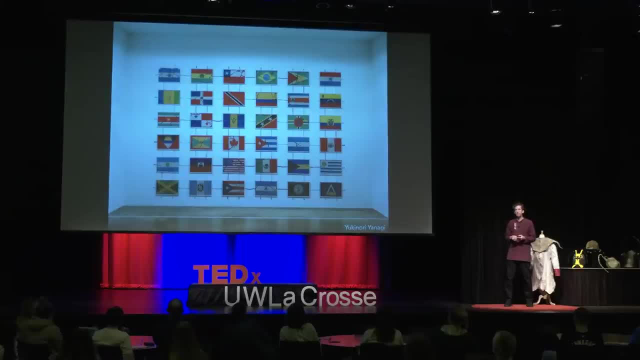 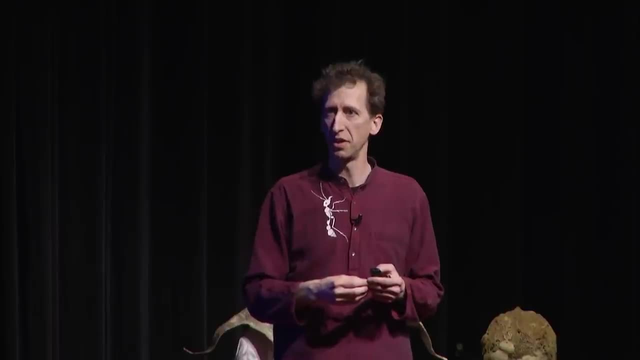 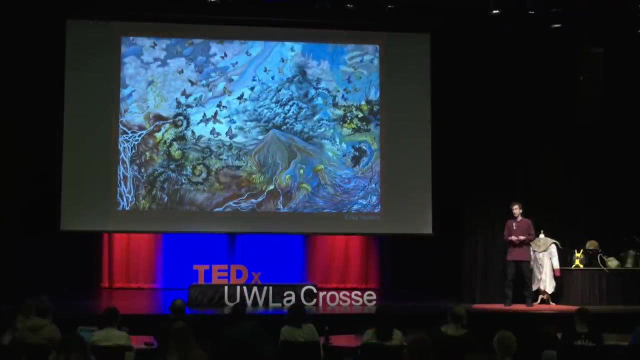 of political boundaries. Oftentimes, art forces us to address challenges, problems in the world. And what is the single greatest tragedy, catastrophe and challenge we face today? It's our wholesale destruction of the living planet. Science is essential, but it's insufficient. 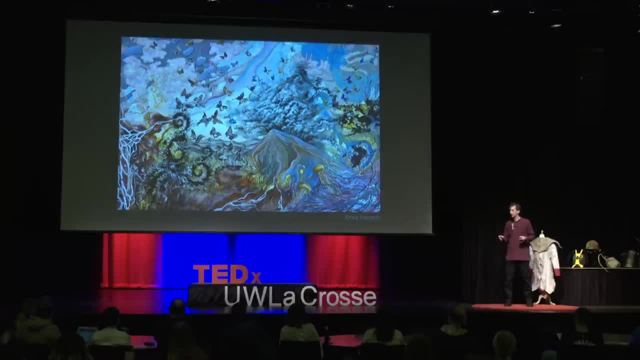 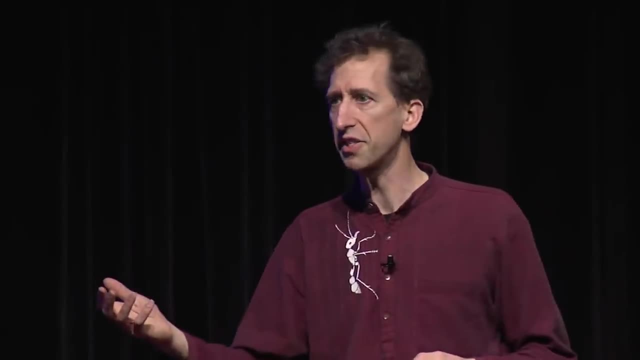 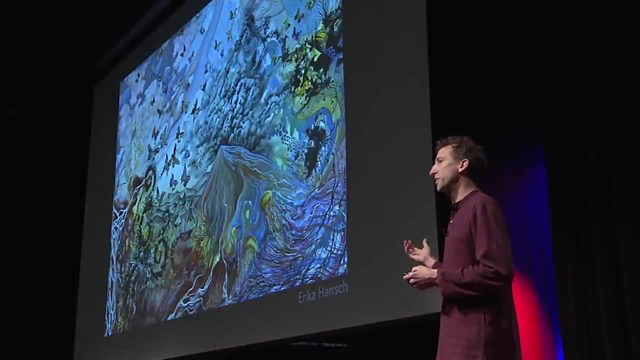 to sway the minds and the hearts of the masses. So we need other mechanisms, we need collective messaging, and art and artists can present a different way to evoke emotions. In this case, Erika Harsh was inspired by witnessing firsthand glacial melting. 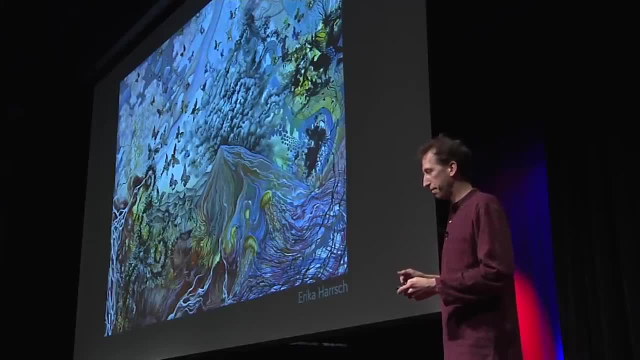 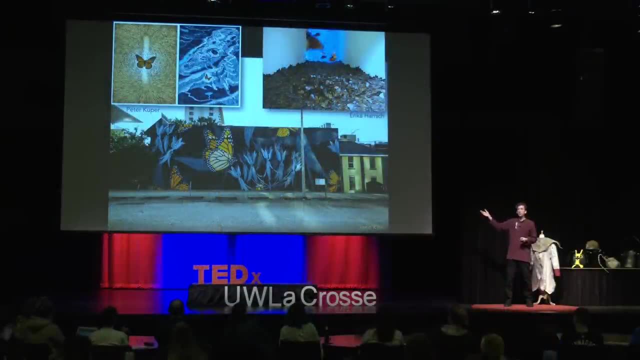 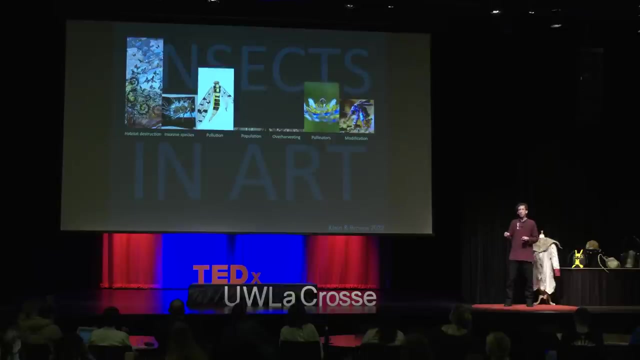 and incorporates insects in her vision. You can look to insects, including our national insect, in terms of declines in numbers, And all three of these artists are commenting on the hazards monarch butterflies are facing. Fellow entomologist Tierney Brocious teamed up with me. 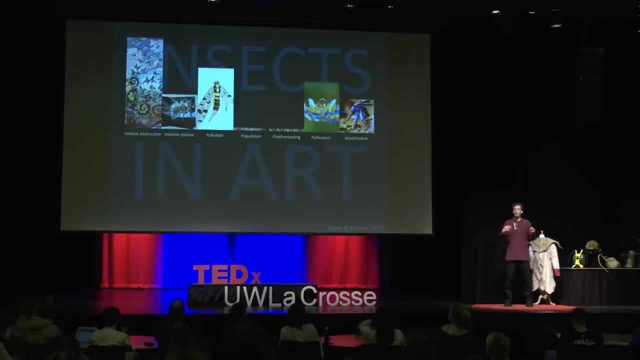 to survey insect art, art that incorporates insects in some way to convey, in this case, messages about human-caused environmental destruction. And you see, these categories are expressed more or less in our surveys. Let me take you on a tour, Starting with habitat destruction. 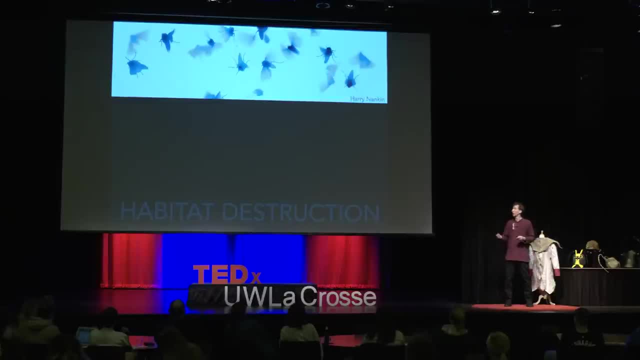 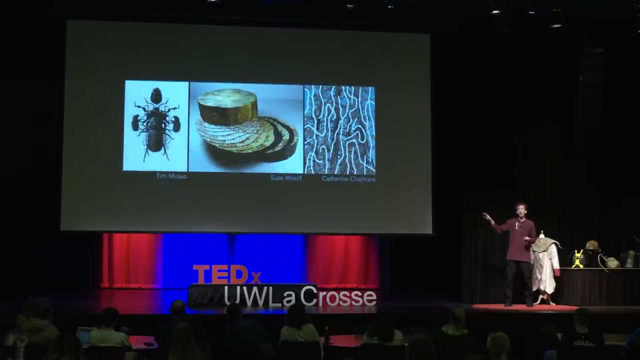 including global climate change, which we're causing. This bogong moth is suffering in Austria, as is this species of moth fashioned in metal and numbered, and each number represents an actual individual presumed to exist in Austria today. These three artists are depicting bark beetles. 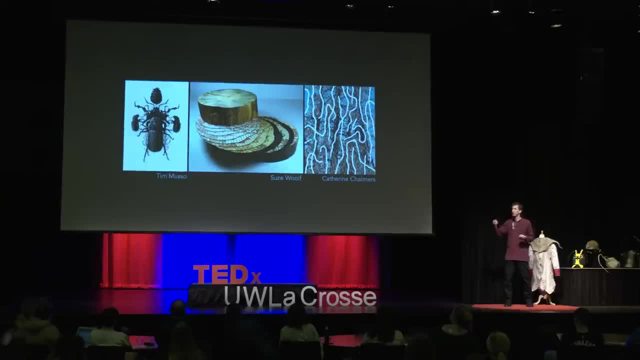 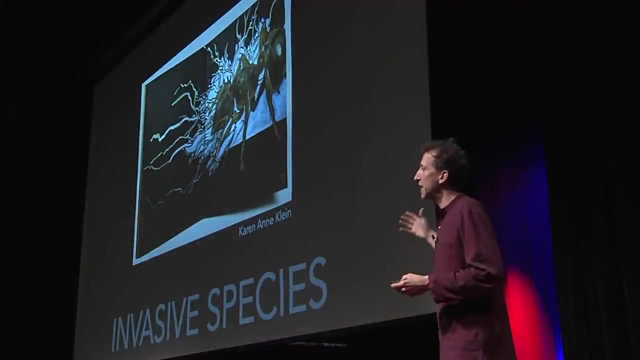 and commenting on forest mismanagement and habitat destruction, facilitating the spread of these bark beetles. Next category: invasive species. Consciously or unconsciously, we spread organisms all over the planet. In the case of the electric ant, it's introduced and it. 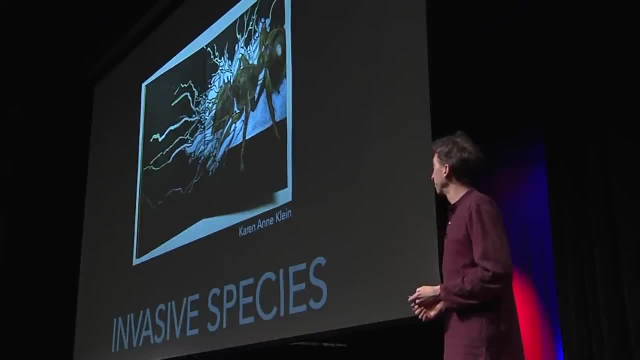 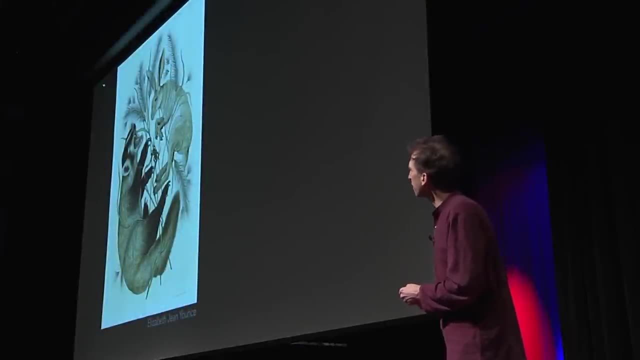 supplants native species, including insects. Sometimes the insect isn't the perpetrator, it's the victim. In the very center here you see that Jerusalem cricket by Elizabeth Jean Younts. This is the victim of buffelgrass, an invasive species. 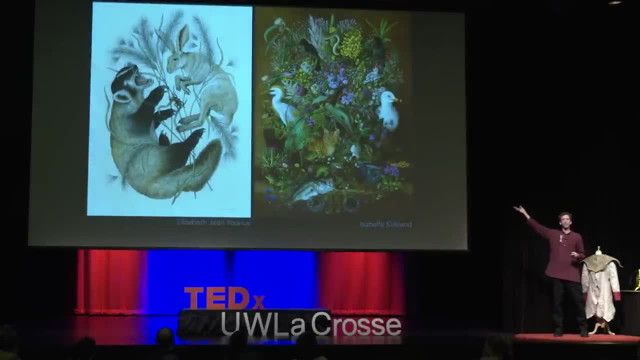 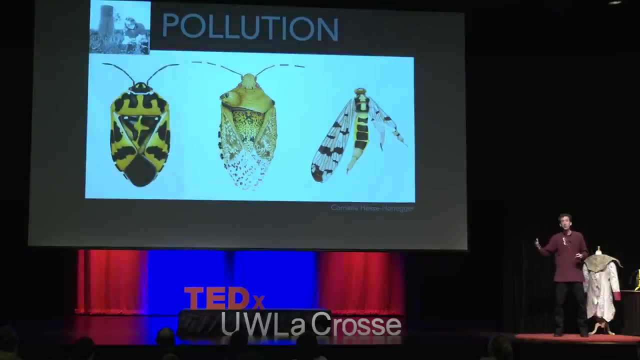 And Isabella Kirkland has collected all invasive species here, including a dozen insect species, each with its own story: Pollution. Cornelia Hasse-Honegger, scientific illustrator, artist, environmental activist, collaborating scientist, looks at insects that are mutated. 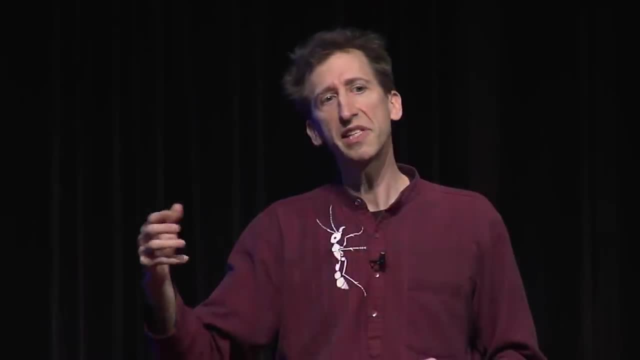 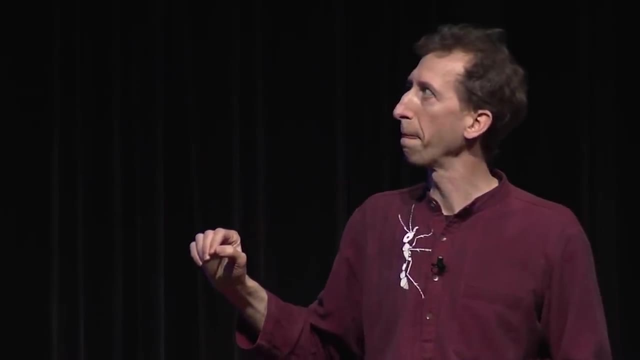 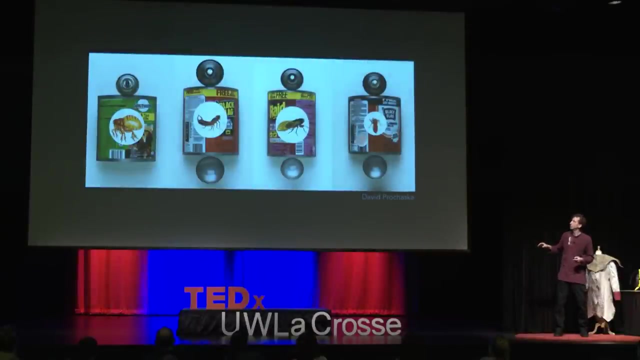 near nuclear power plants, Even the safest, cleanest ones, she claims, are mutating insects in their vicinity. David Prochaska paints insects on canisters of doom, And then we've got the category of over-harvesting, And you might just walk by. 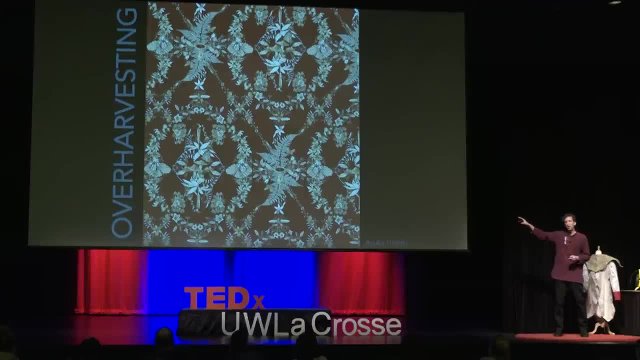 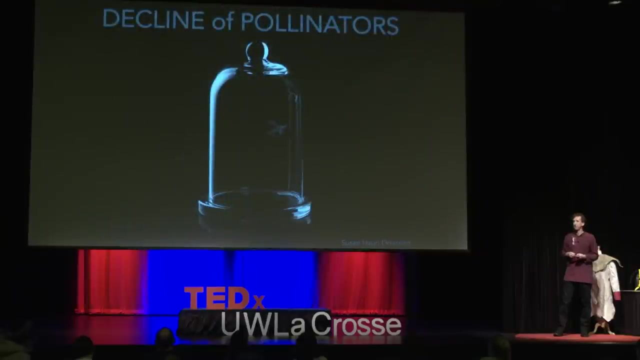 Asuka Hishiki's wallpaper here, not noticing all of the human-induced atrocities represented by insects and other species that are declining rapidly in numbers. Now we move into a couple of categories that are more insect-specific, like the decline of insect pollinators- Here a wasp. 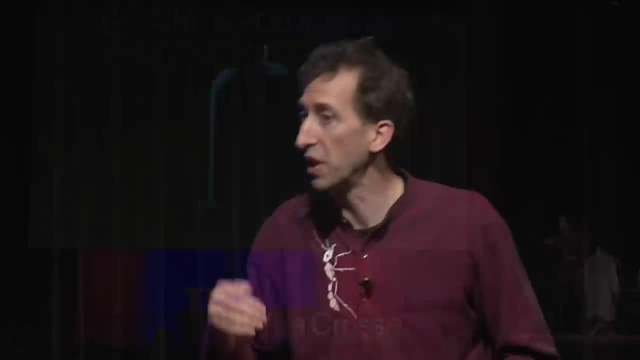 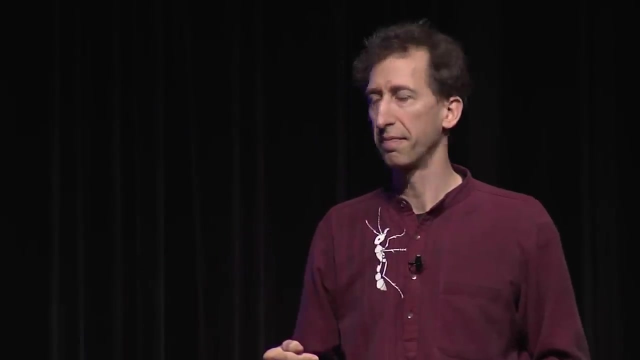 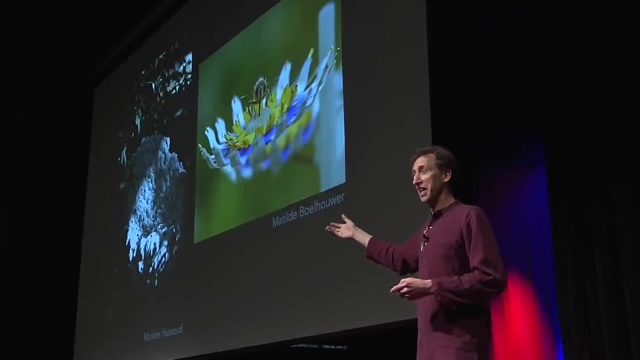 etched on a glass bell jar is disappearing because it's a specialist pollinator on a plant that's vanishing. Here we've got two artists that are going to the lengths of offering homes, as well as food, to urban insect pollinators. Desperate measures. 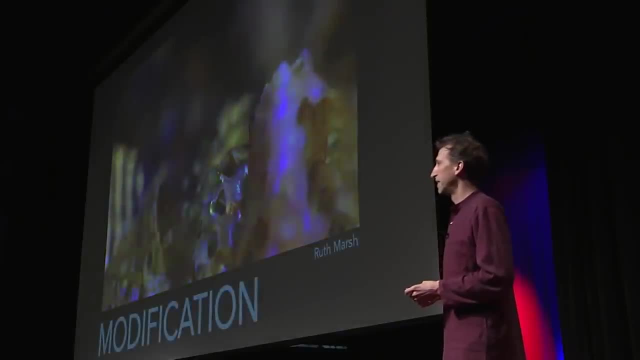 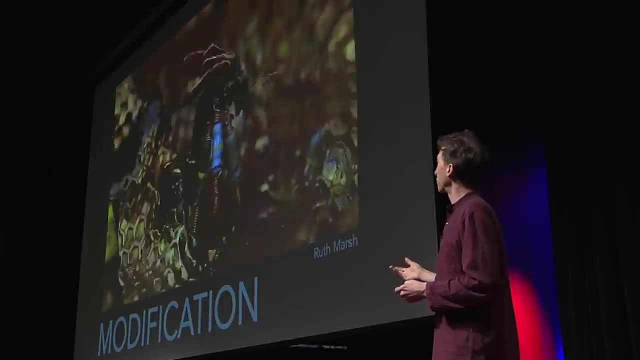 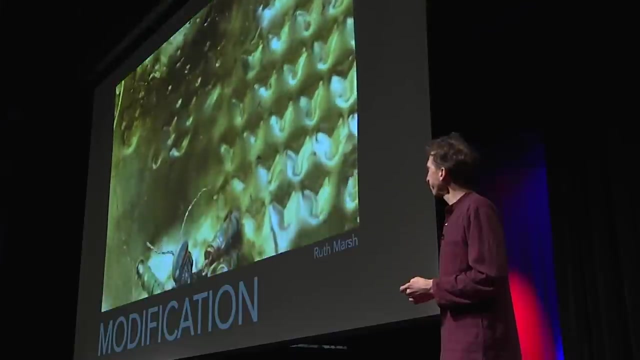 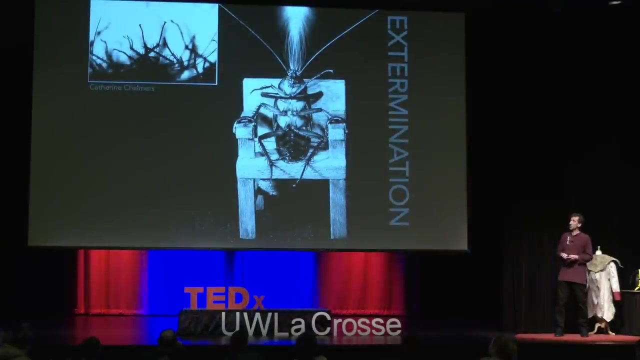 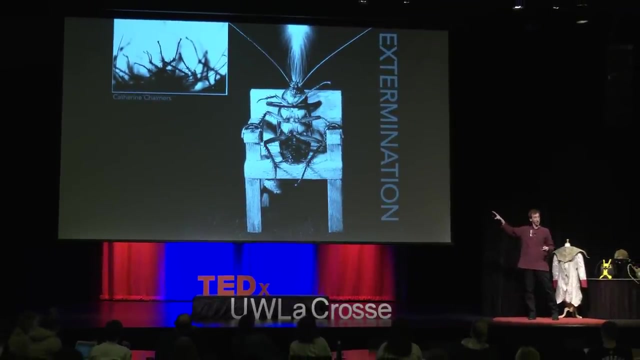 Then the category of intentional insect modification, including genetic modification- Ruth Marsh produced this cyber-hive, an animation with cybernetic bees. And finally, intentional extermination of insects. And while no American cockroach was harmed in the production of these videos, 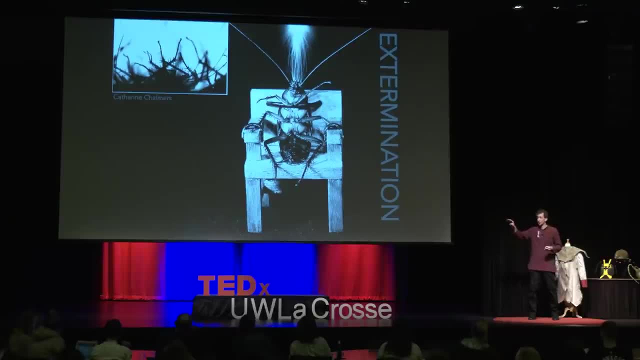 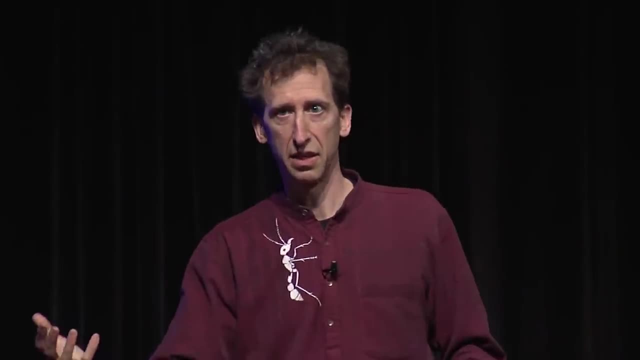 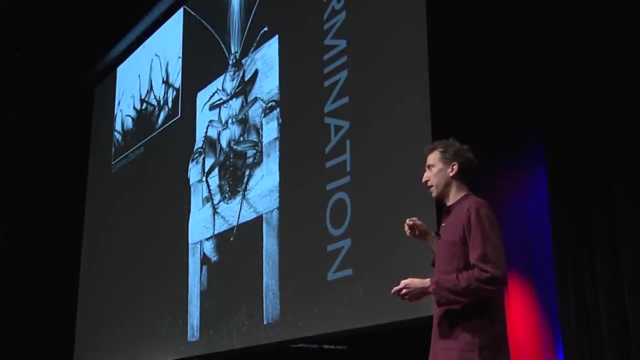 and stills produced by Katherine Chalmers for an execution series. it's very difficult for us to not empathize when we look at these inhumane human practices of execution or torture, Which is interesting because the focus is an insect that humans typically revile. 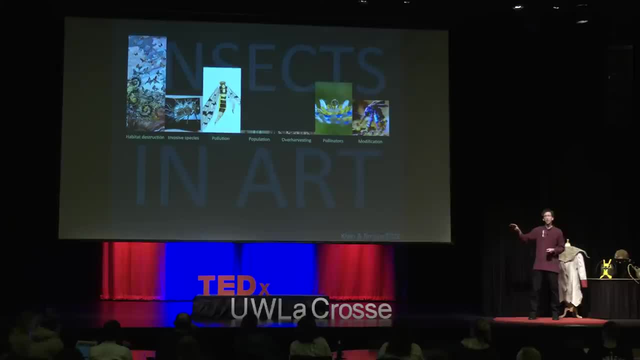 So if we step back and we look at these human induced categories of environmental destruction, we see- as artists, as scientists, as humans- opportunities. Look at the center there: Population That represents human population growth And in our survey we saw almost no. 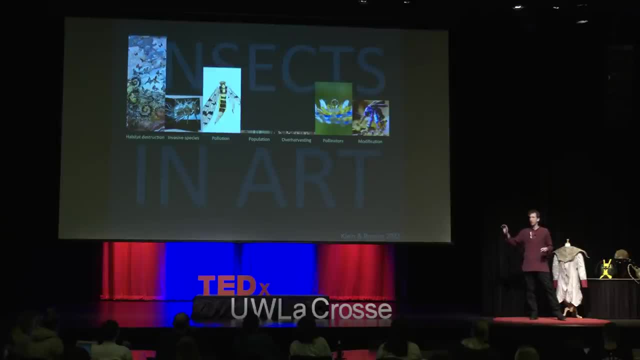 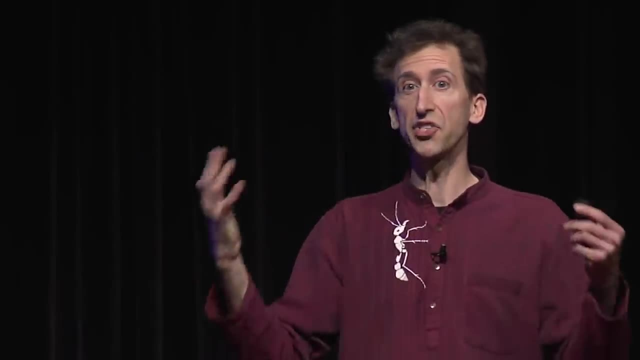 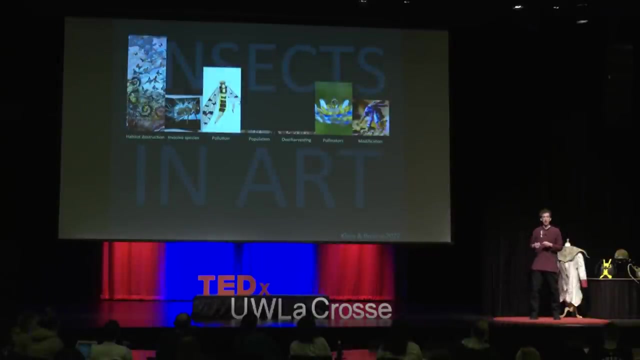 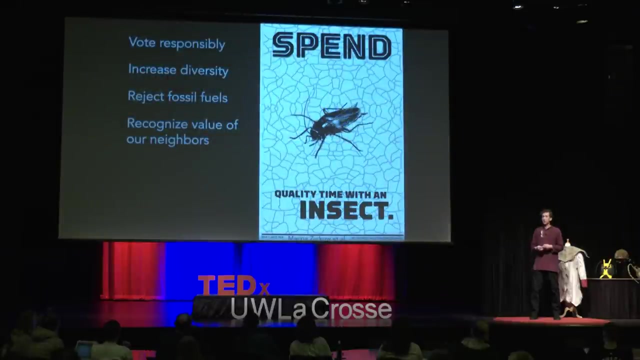 insect works that explicitly represented human population growth. But that very process of expanding exponentially our numbers exacerbates, is instrumental in affecting all of the other categories. There's a problem here And we need to address it at every level. But what? 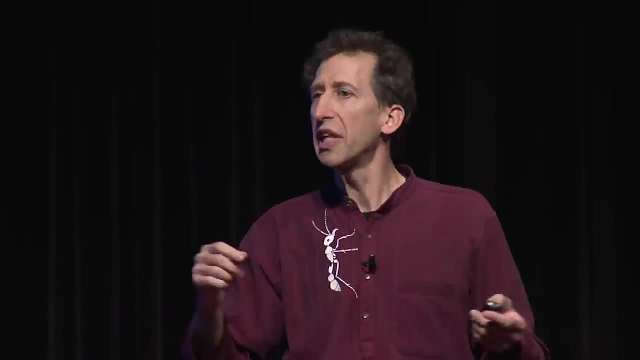 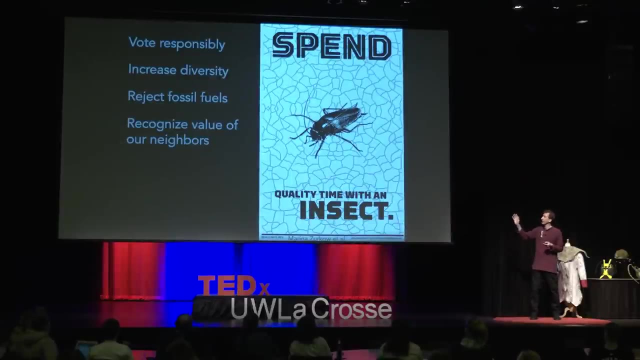 can you do? What can we do? There are actually a lot of things we can do. I've put a very short list, which we could expand all day. Voting responsibly is key, Increasing diversity, including in your own yards, As well as rejecting. 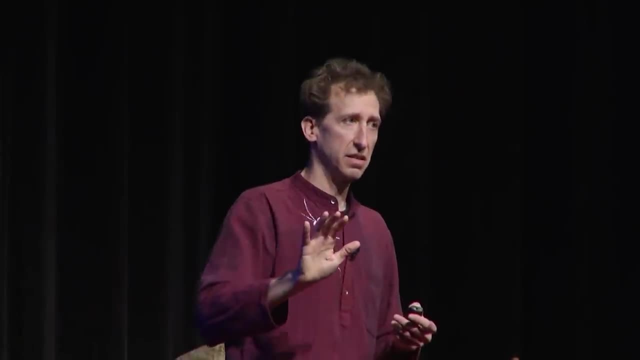 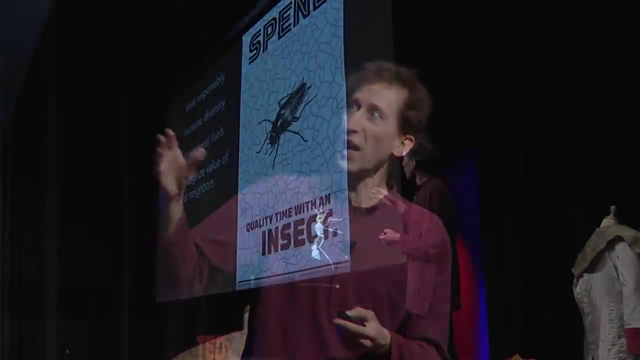 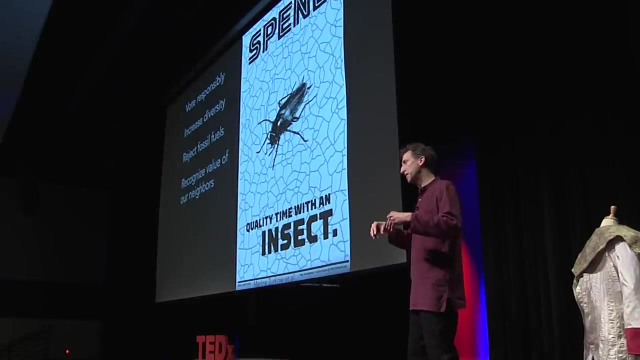 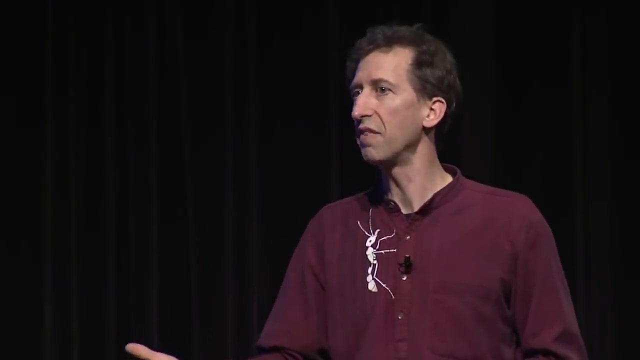 fossil fuels, Divest, Reduce your reliance on fossil fuels And simply recognizing the value of our neighbors. So if we better understand that we're a single species interconnected with multitudes, maybe we would conduct less atrocious behavior leading to biodiversity or life's diversity declines. 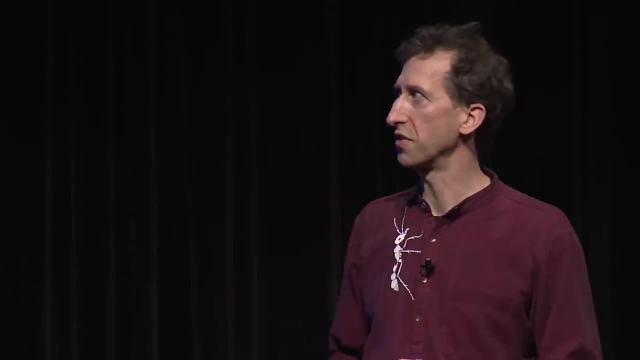 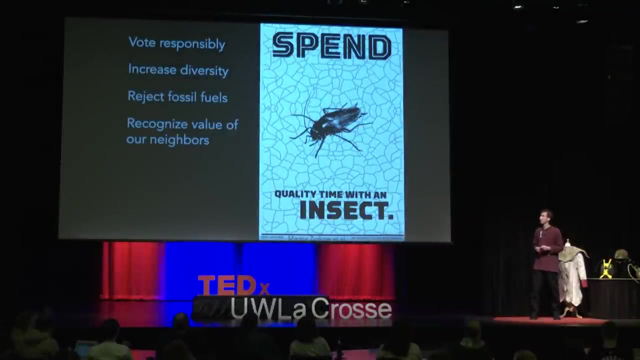 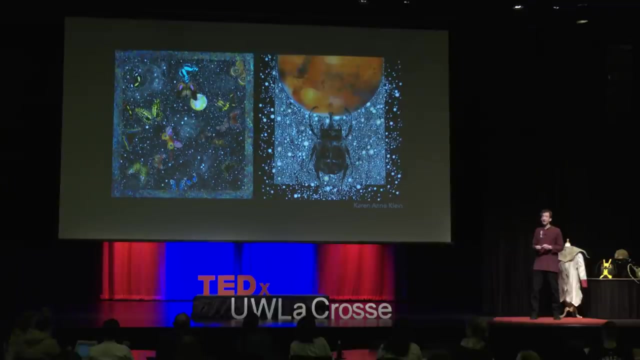 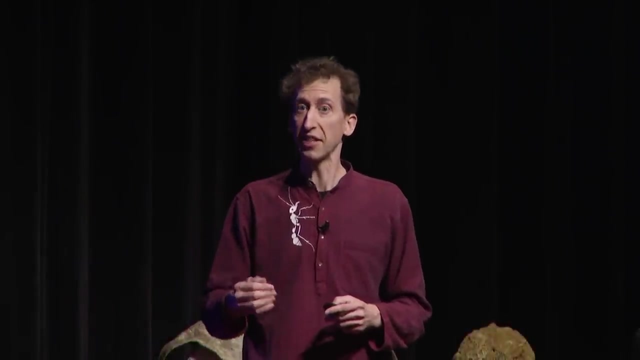 And affect all of those categories of destruction. Lastly, we should spend more time with nature, Quality time with an insect. We can appreciate insects through art, as my mother does Again. art can uniquely evoke emotions and potentially enact change, And insect art is included. 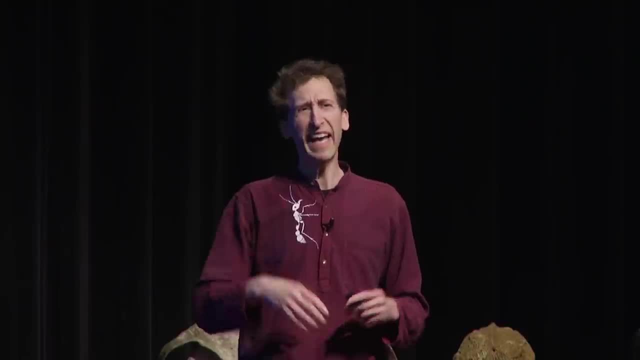 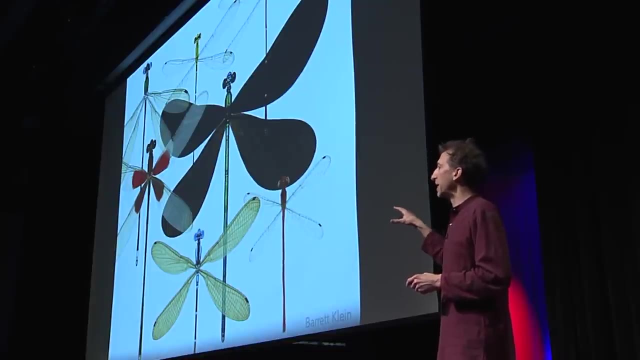 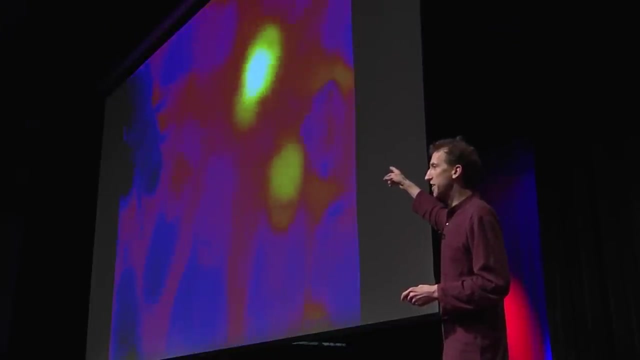 in that We can find any group, say, for example, a diversity of damselflies, and look at the beauty in shape, form, color and behavior. Or we can focus on one species, like this honeybee waggle dancing to communicate. 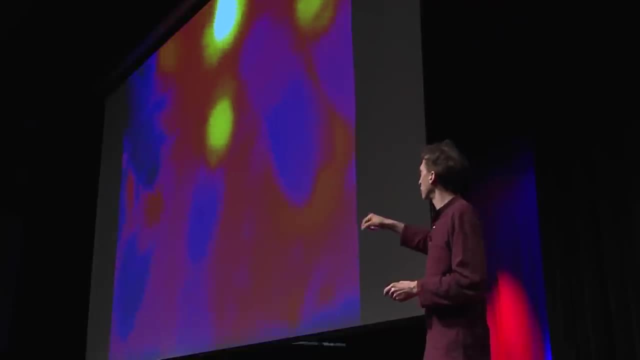 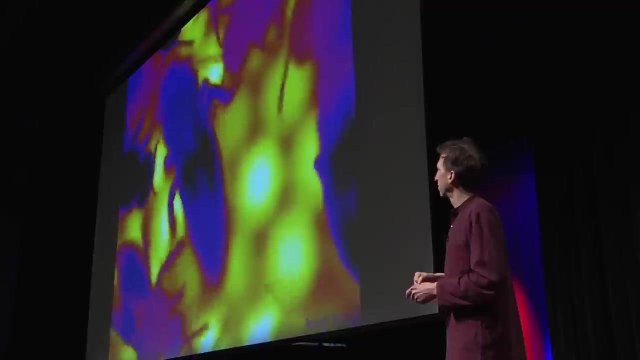 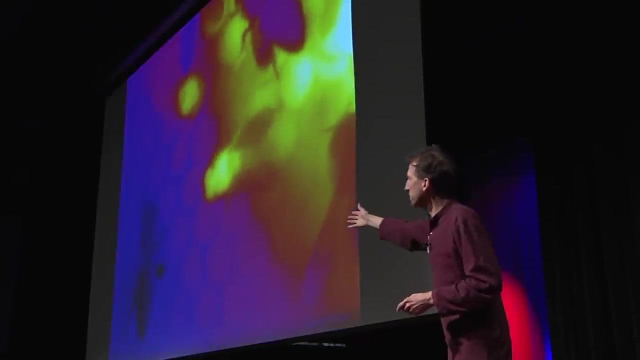 distance and direction, to a distant food source, to her nestmates, Or this one fanning her wings to cool down the nest, This queen tended by a phalanx of nurse bees. All of these activities, including sleep, happens in one colony.